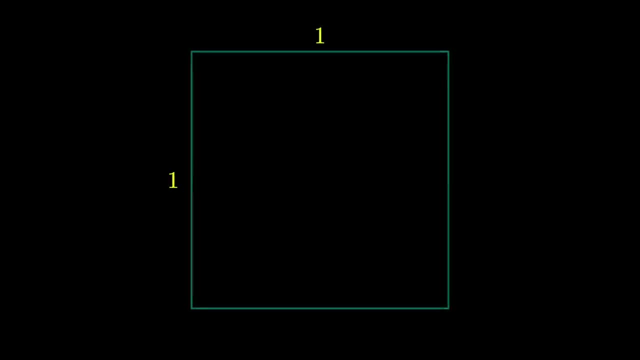 version of the problem. Draw a unit square and its diagonal. Let's use a similar process to try to figure out what the length of this diagonal is. If we follow the perimeter from one end to the other, we see that this path length is 4.. 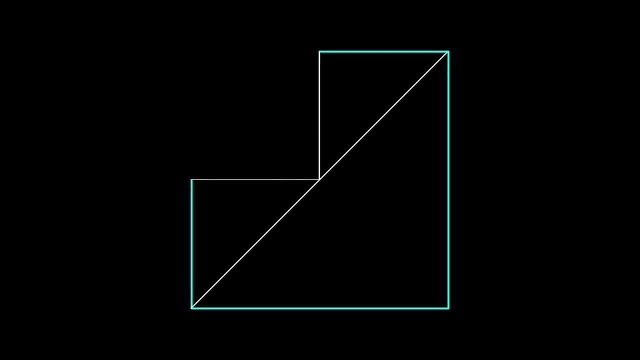 Cut out the upper corner of this region and travel the perimeter again, we'll see that this again is path length 2.. Repeat over and over, out to infinity: the length of the path is still 2.. And our path approaches the path of the diagonal. So should we conclude? 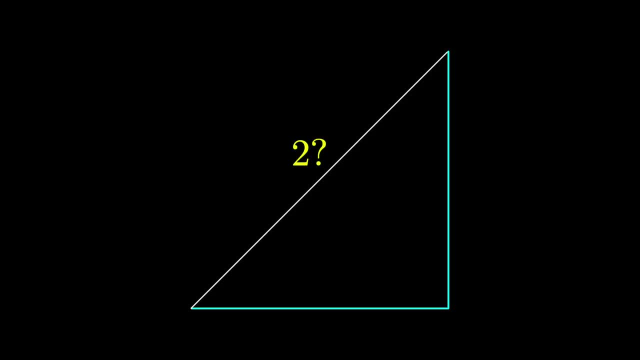 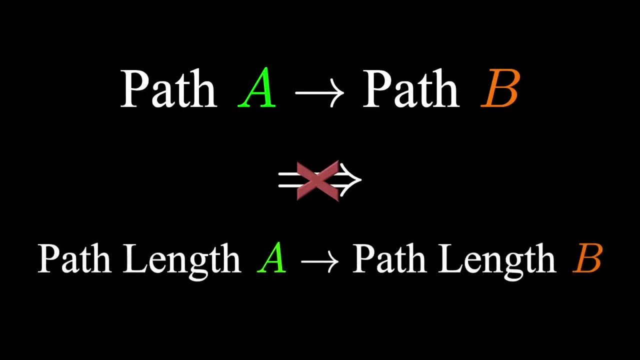 that the length of this diagonal is 2?? And the answer is, of course, not. The problem with this is that just because one path approaches another, it doesn't mean that the length of the path approaches the length of the other. How can we mathematically show this? We can. 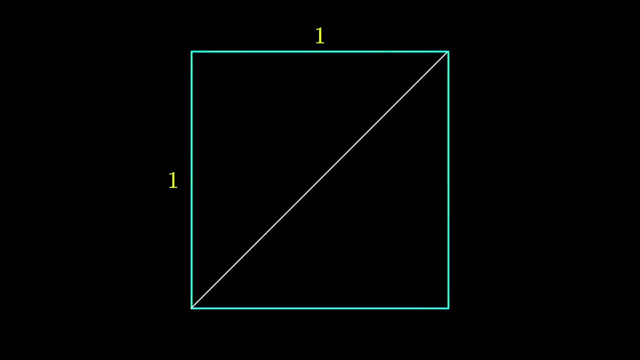 say that the staircase path approaches the diagonal by looking at the area between them. If this area shrinks to 0, we'll say that the staircase path approaches the diagonal path. Let n be the number of iterations in this process. So when n equals 1, we have one step: making a triangle with base 1 and height 1.. 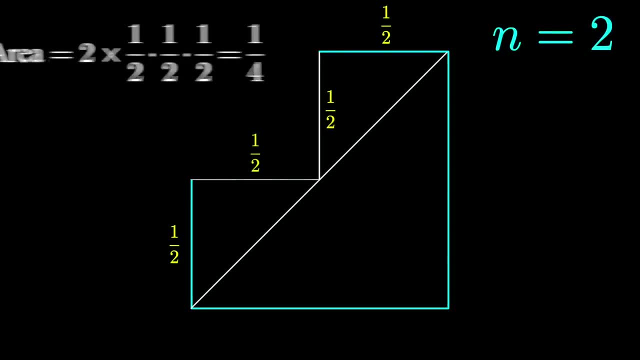 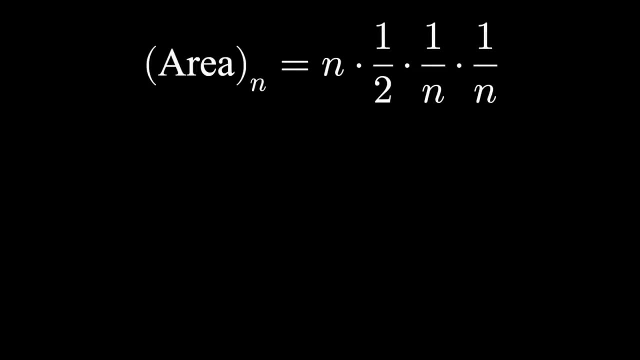 When n equals 2, we'll have two steps with base 1 half and height 1 half. So for a general n times 1 half times 1 over n times 1 over n, we have n triangles each with area 1 half base times height. 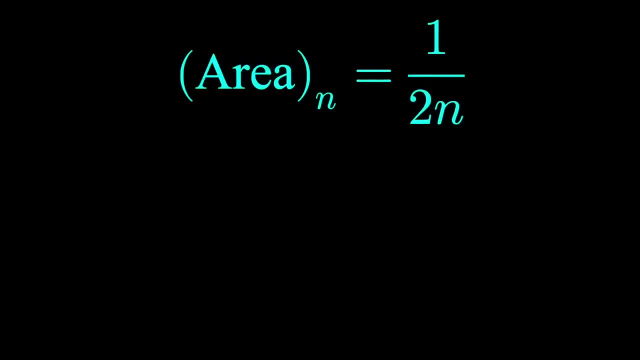 In other words, the area of the nth iteration of our process is 1 over 2n, And we can see this area shrink to 0 by taking the limit out to infinity. Thus we conclude that the staircase path does indeed approach the diagonal path. 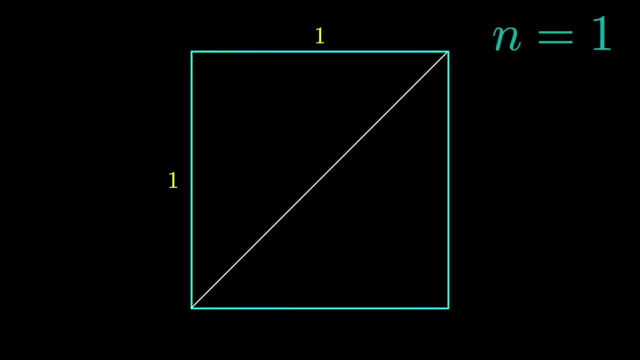 However, if we do a similar process for the lengths of these paths, starting at n equals 1, the staircase as a path length is 1 over 2n. At n equals 2, the staircase has path length 1 half plus 1 half times 2 is 2..